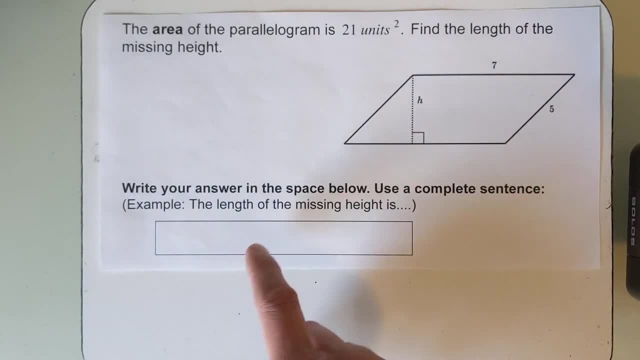 Make sure you do write your answer as a complete sentence down here in the space. So, for example, the length of the missing height is blank and you're going to go ahead and write it there. Remember, you do not have to have the correct answer. That is totally okay. 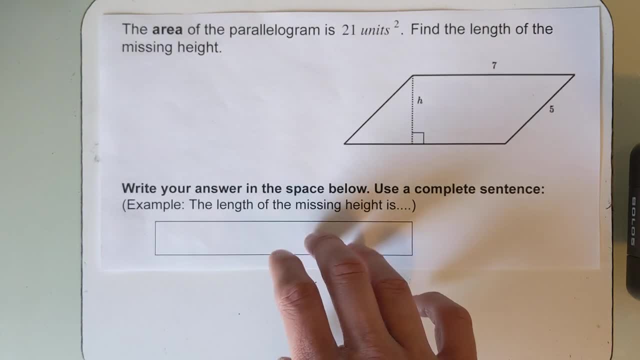 but take as much time as you need to have something written there and it has to be a complete sentence. Again, real focus today on complete sentences and writing in those complete sentences. Go ahead and pause and resume when you're ready. Pause again in the next five. 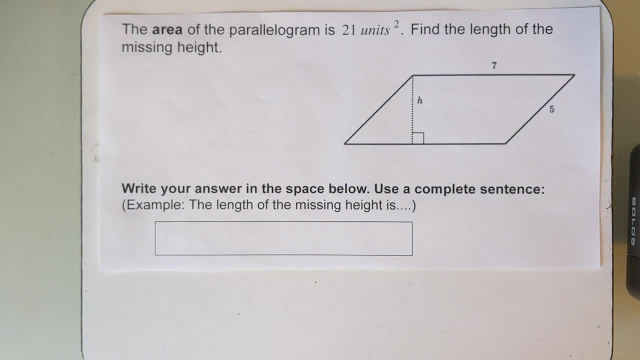 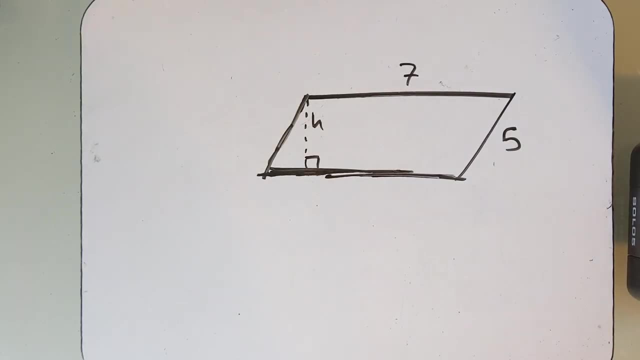 four, three, two and one. So let's go ahead and take a look at this. I just went ahead and drew it on a different side here, or just a different area. So if you want to redraw it, you totally can. That's all. 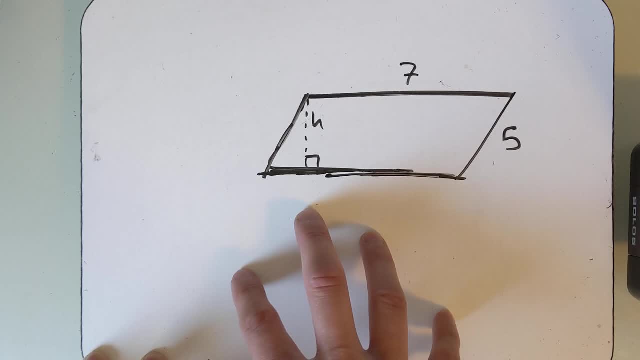 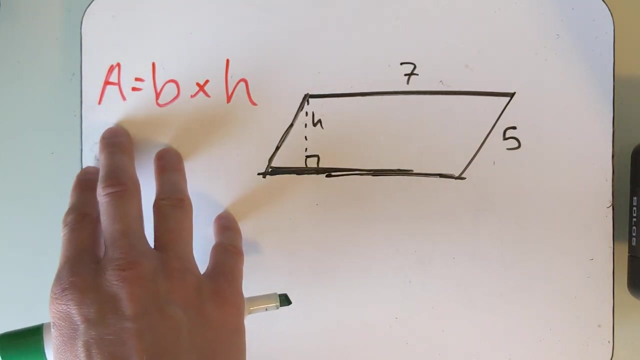 right, I'm just doing this so it's a little easier to look at. So if we look here, first off we remember that yesterday's lesson we learned that area, our formula is area, is going to be the base times the height. okay, So all we need to do is figure out if we 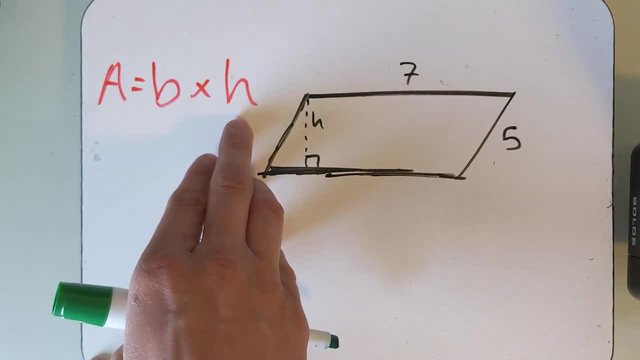 know our area, what is the base and what is the height, right? And some of that information is already given. So, for example, we know the area is 21 square units, right, We know it's 21.. So I'm. 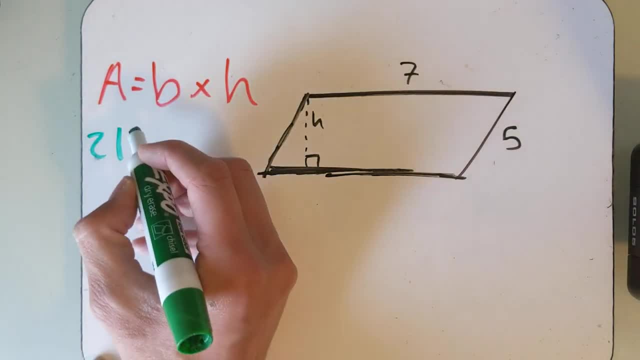 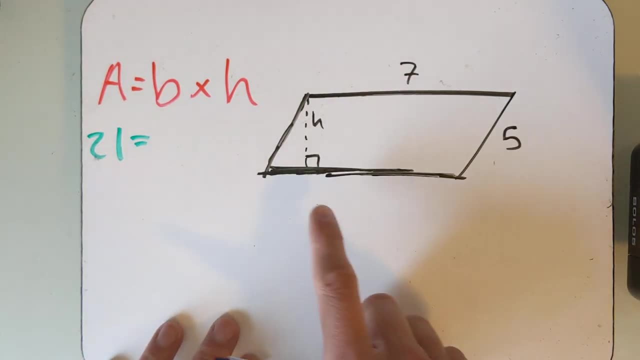 just going to go ahead and write the number 21 under here. So we have 21 is equal to. and let's look at our base and our height and just write those numbers down. So our base is down here. It doesn't have a number here, but we know opposite sides of the parallelogram are equal. 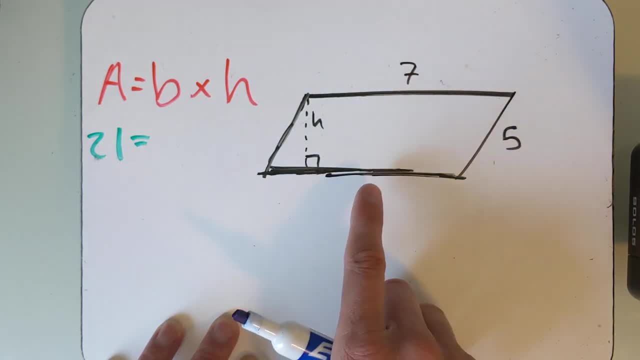 We've talked about that quite a bit this year. So that means if this side is 7, so is this side. So our base is just 7.. So we have: 21 is equal to 7 times what number. So this is really the only. 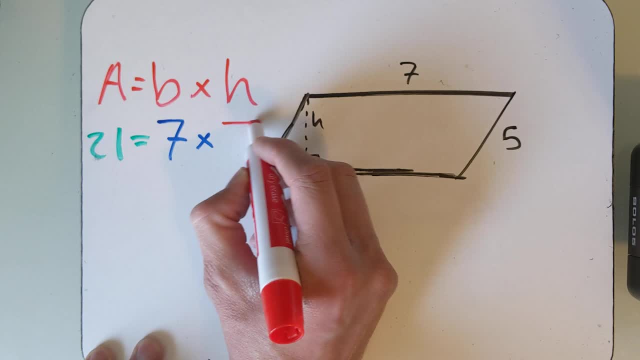 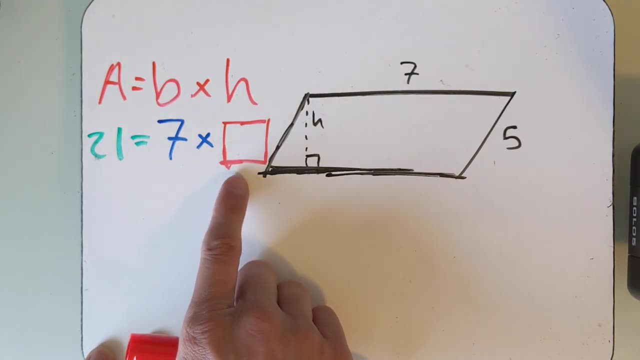 thing that we need to solve for at this point is: 21 is equal to base times, or sorry, 7 times what right? So, again, just with basic math facts, we know that 7 times 3 would give us 21,. 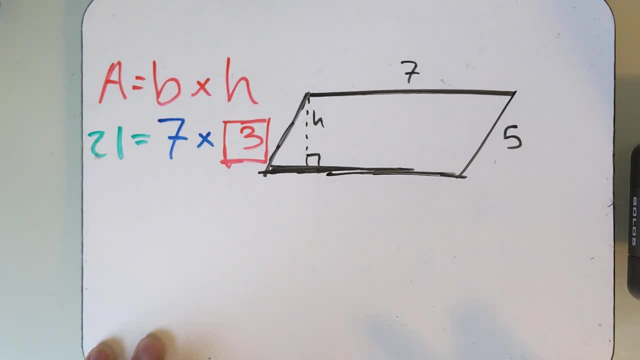 so I'm just going to go ahead and write a 3 in here and that's our answer. It's that easy. This 5 is just extra information. You don't even need to use it. They're just trying to confuse you here. So our height is 3.. We don't have any units here, so we would just write that the length. 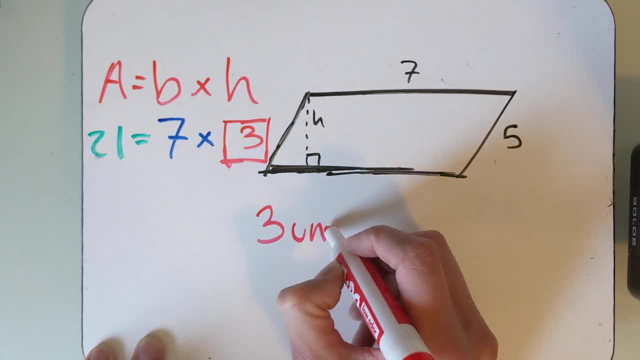 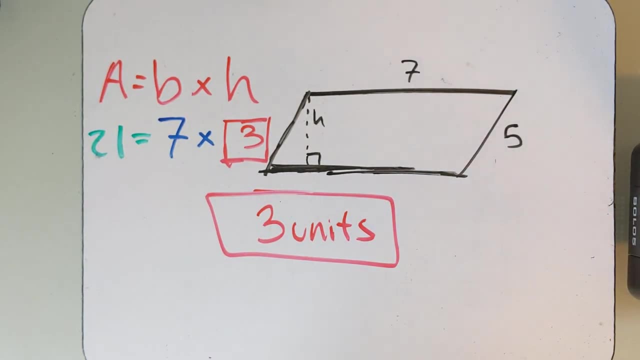 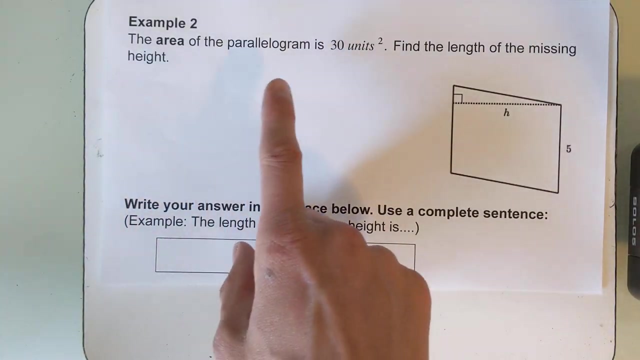 of the missing height is 3 units, and this is our final answer. That's it. Let's go ahead and do one more, just to make sure that we fully get that. I'm going to go ahead and get set up here. This question says the area of the parallelogram is 30 square units. Find the length of the missing. 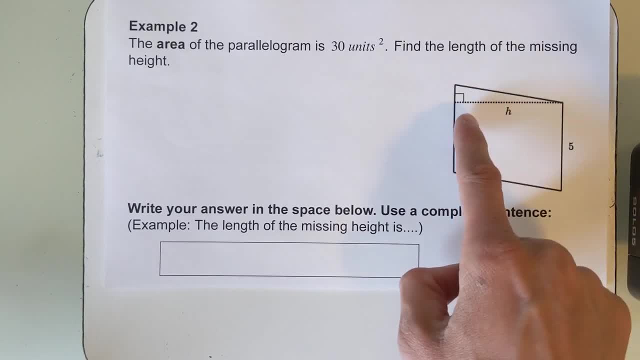 height. So if we look here, even though it goes left to right, they still label it as height. so we're just going to call it the height, and we know this side over here is 5.. So, remembering again that the area is equal to the base times the height, I'm just going to go ahead and write. 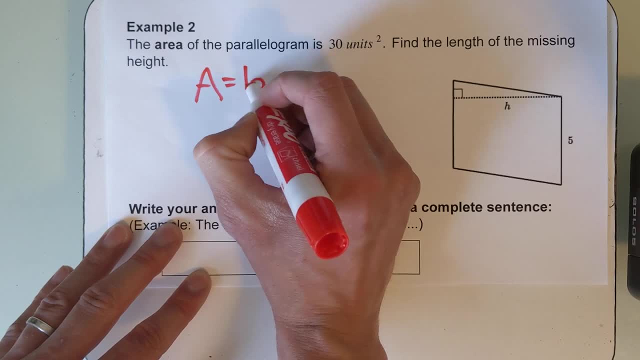 on here for now. so I'm going to rewrite that formula: Area is equal to base times our height, So we know the area is 30.. We're going to go ahead and write that formula Area is equal to base times our height, So we know the area is 30.. 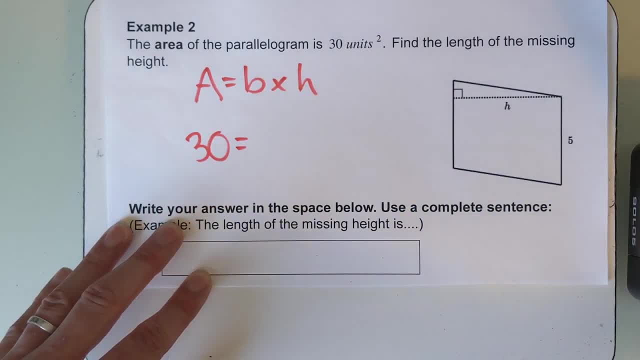 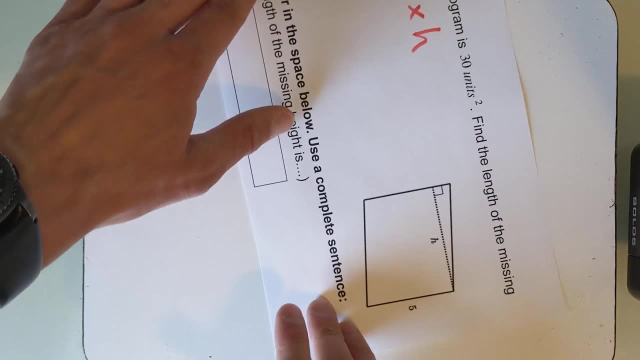 Square units. So we're just going to write a 30. there is equal to the base, right, And we will call this the base here, just because they call it the height. It's okay, Even if we just rotate it, it still gives us the same answer or the same number. So we have a 5 times the height. 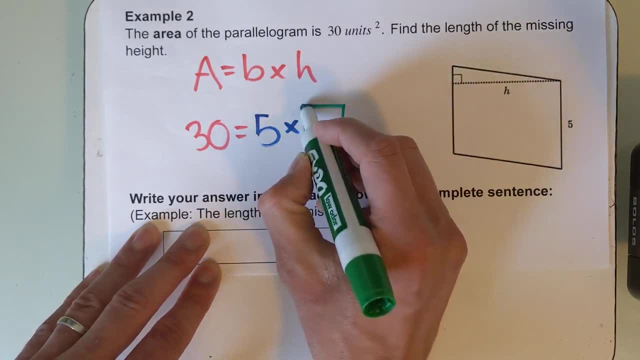 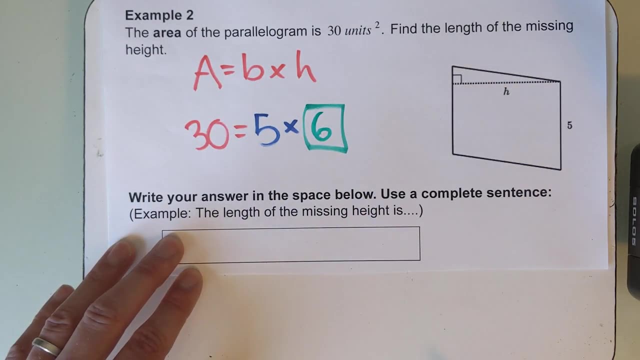 which is we don't know. So just figuring out 5 times what number is going to give us that 30. Here we would go ahead and say that it's 5 times 6 is going to give us that 30. So our answer: 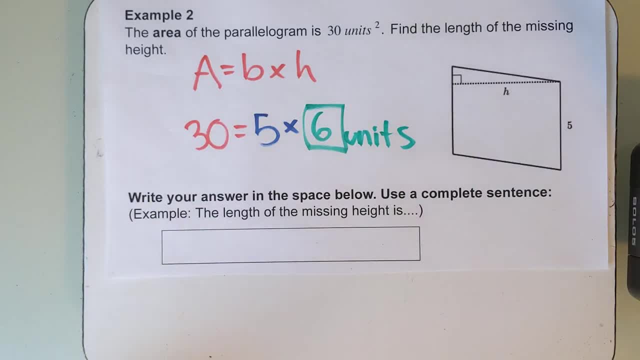 is just 6 units. So the height is equal to 6 units And of course we would use a complete sentence here by saying the length of the missing height is 6 units. Go ahead and take a minute here, to go ahead and type in your full, complete sentence of your answer. 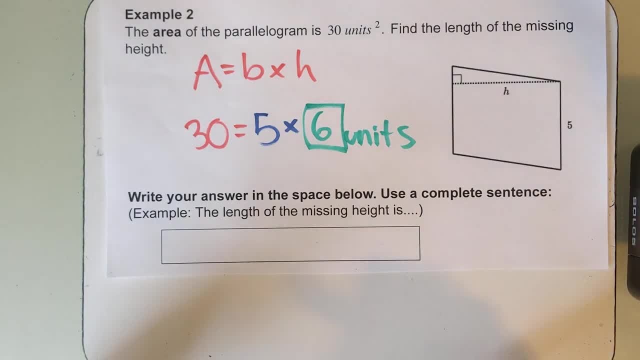 And then we're just going to go ahead and look at question one, Question one. you are going to start on your own and you'll solve it. So we're going to go ahead and look at question one And then we're going to solve that, And then you'll come back together, resume the video, just to check your. 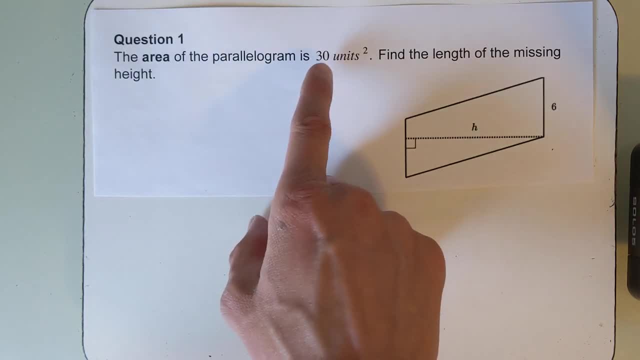 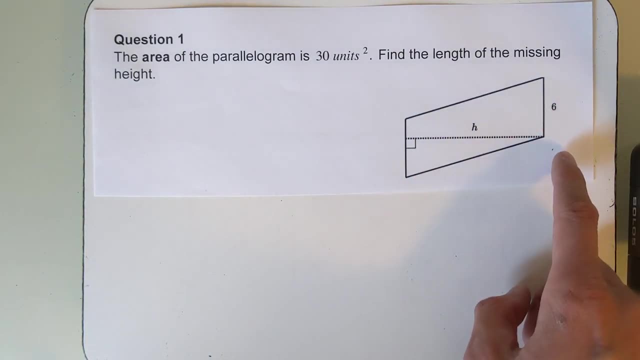 answer. So here, question one: it says the area of the parallelogram is 30 square units. Find the length of the missing height. So we need this height. We know what the base is going to be, Again, remembering that area equals base times height. Go ahead and pause and then resume when.